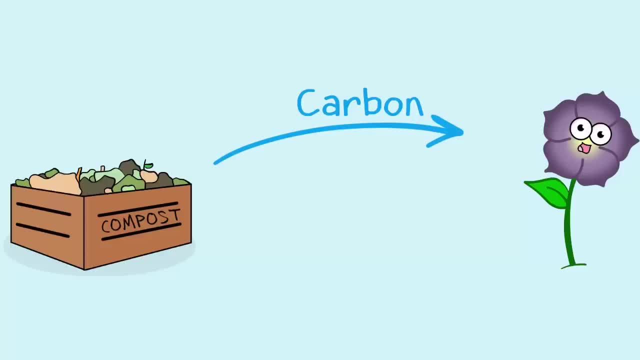 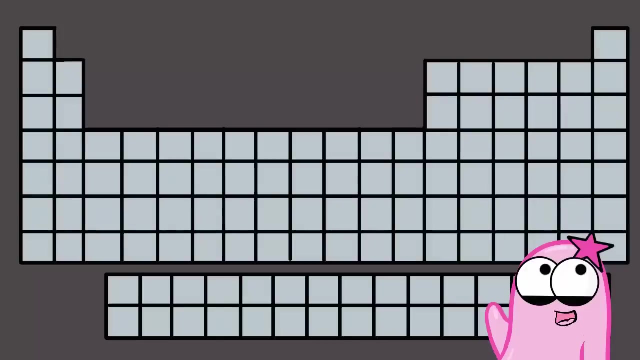 supply plants with that are so important: Carbon and nitrogen. We're going to spend some time talking about these two elements and their cycles, because both of them are so important for life. With so many incredible elements on the periodic table, we don't know if it's really fair to have a favorite, but we do. It's carbon, Sorry, nitrogen. 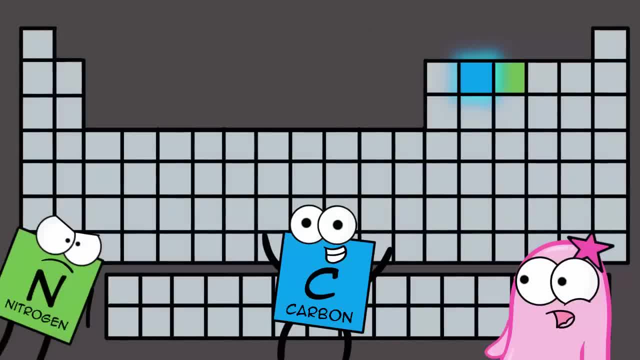 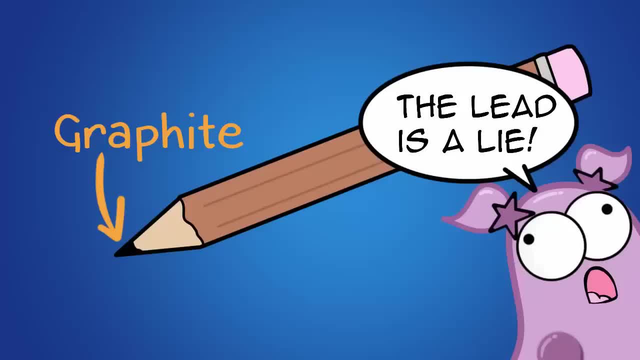 you're cool too, but why the love for carbon? Well, we really love how versatile it is. In one form, it could make up your pencil lead, which really isn't lead at all. it's graphite. It's a form of carbon. In another, 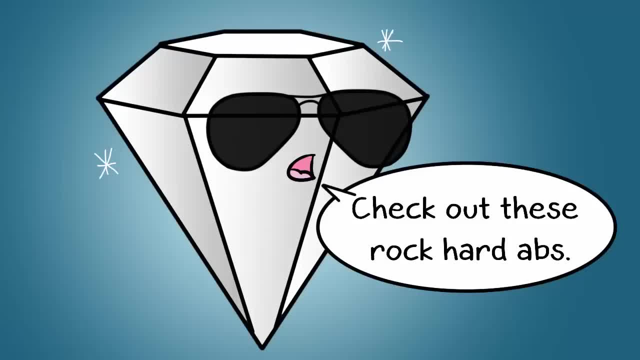 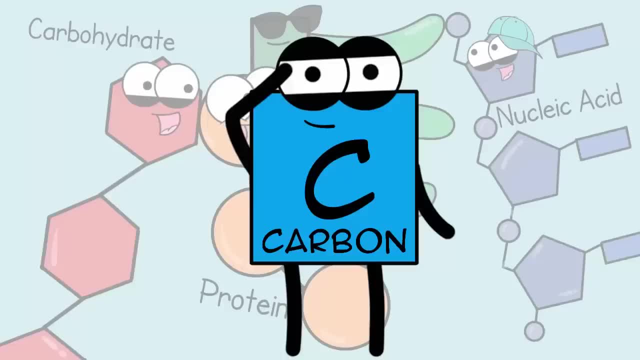 form, carbon can make up one of the hardest substances, diamond. The big four- biomolecules, carbohydrates, lipids, proteins and nucleic acids- they all have carbon. In fact, molecules that contain carbon are known to be organic molecules. 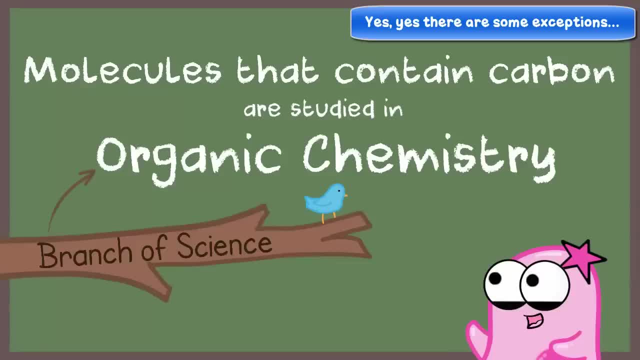 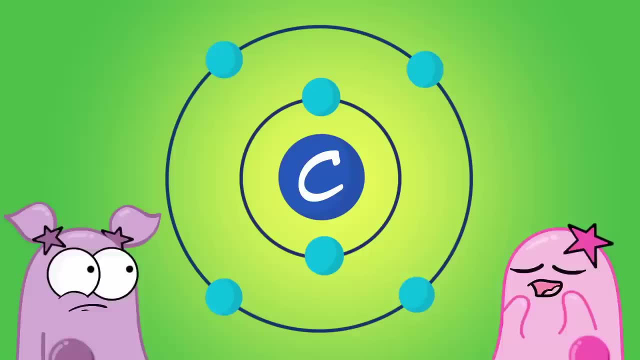 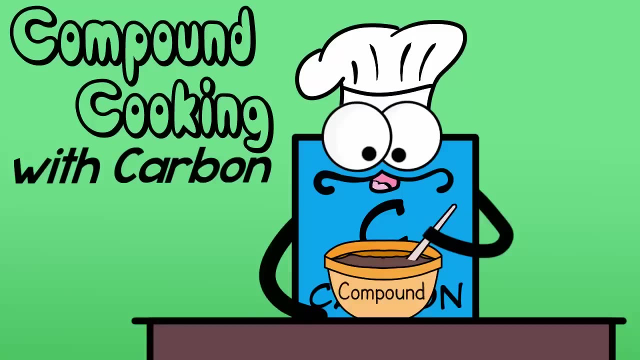 Organic chemistry is a branch of science that studies the interactions of molecules that contain carbon. Just look at this carbon atom. Just look at it. It has four valence electrons, and carbon has the ability to form tons of compounds. Carbon is a building element. 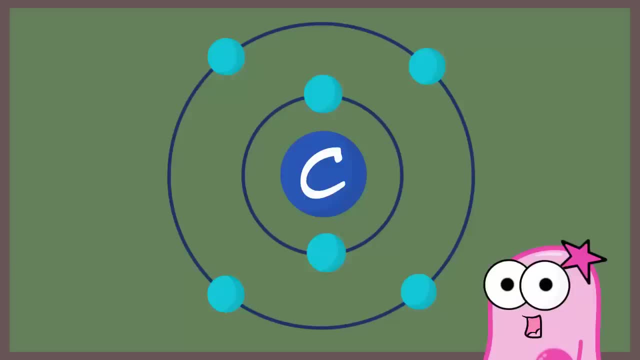 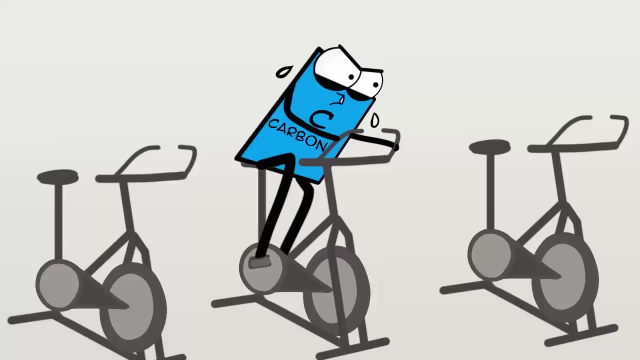 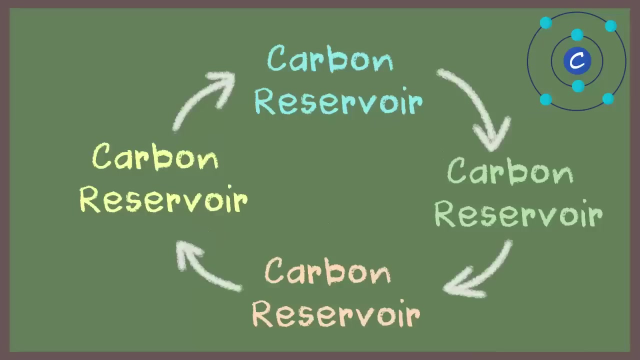 in life for this reason. Well, now that you get the point on how important carbon is, let's make sure we understand how we get carbon. That means we need to take a look at how carbon is First. it's important to understand that there are carbon reservoirs, basically areas where 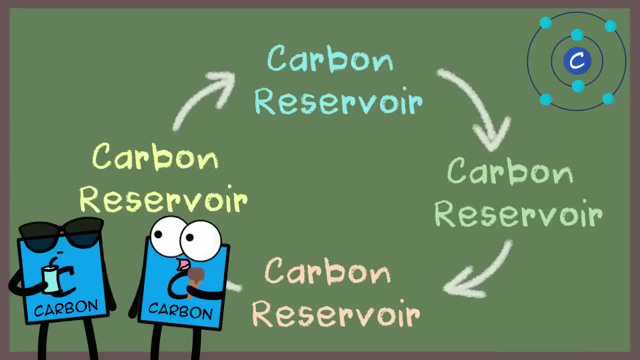 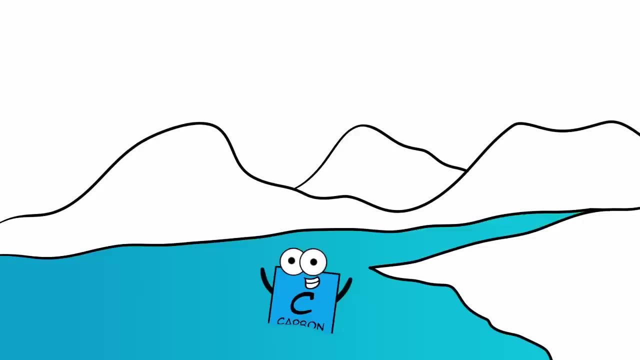 carbon can be found where carbon is hanging out, And the carbon cycle is a cycling among these reservoirs. So here are some major examples of where carbon is found. Carbon's dissolved in the ocean. it's in rocks, it's in fossil fuels. it's in living organisms. it can be found in the 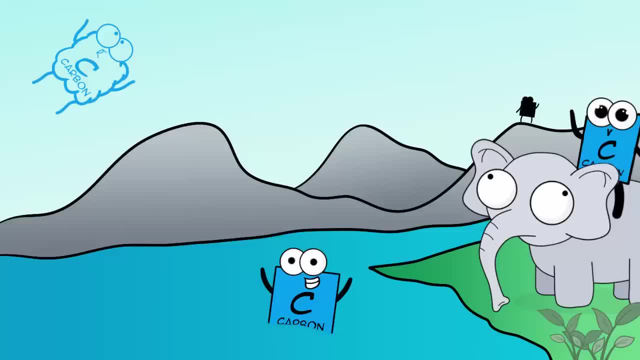 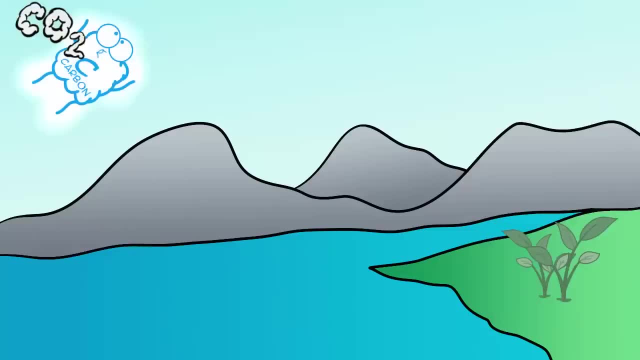 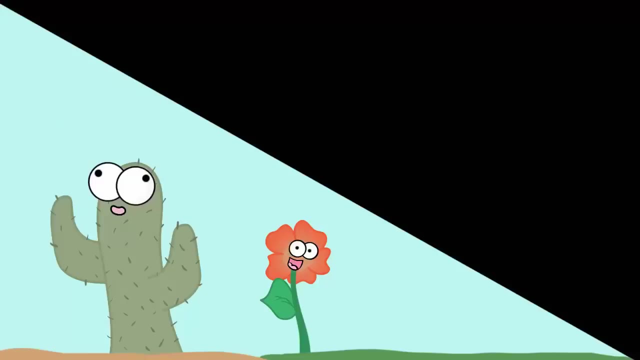 atmosphere. So the idea is to understand that carbon cycles among these reservoirs. Now our time is limited, so let's take a look at one pathway. Consider carbon dioxide in the atmosphere. It's taken in by organisms that perform photosynthesis. This may be plants, it could be algae in the oceans or lakes. The carbon becomes a part of 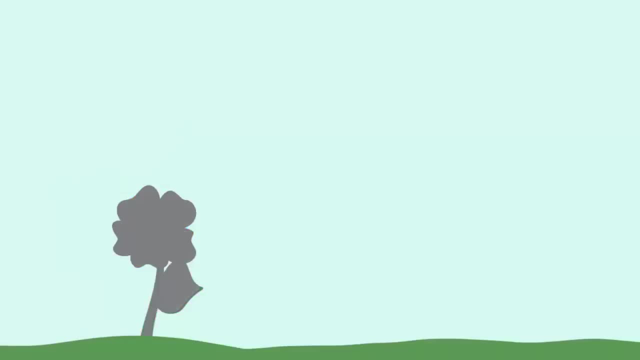 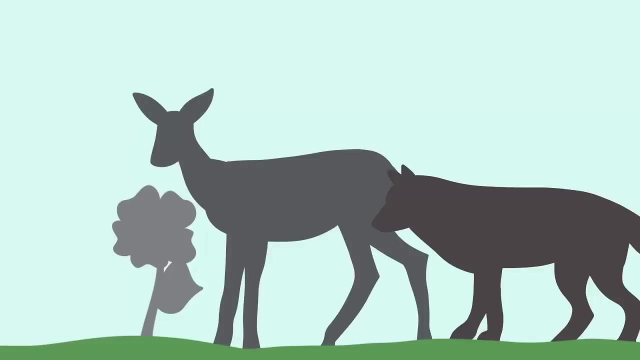 that photosynthetic organism. If the photosynthetic organism is eaten by an animal, it becomes a part of that animal too, And the animal that eats that animal- Both the plants and animals- do something about it. So let's take a look at one pathway. Consider carbon dioxide in the atmosphere. 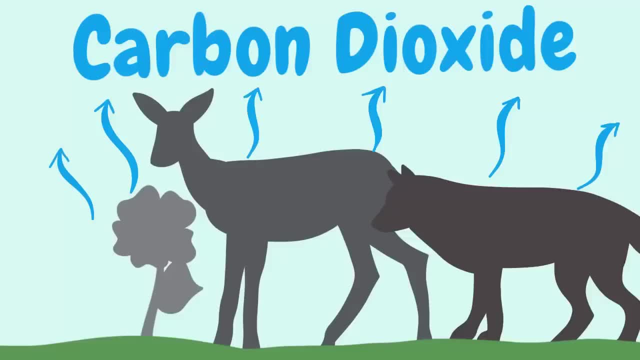 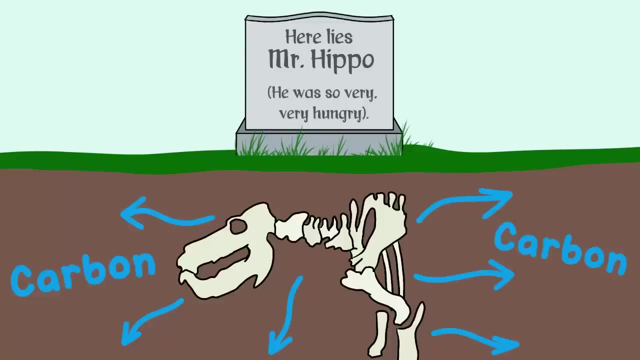 cellular respiration, which releases carbon dioxide. When the plants and animals die, the carbon they contained can be stored in sediment And over a long period of time- a long, long period of time- they can even be converted into fossil fuels. 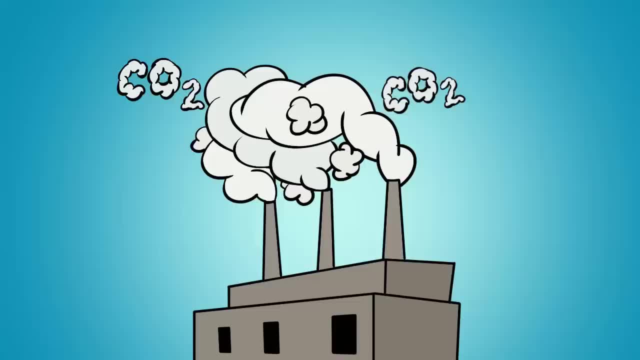 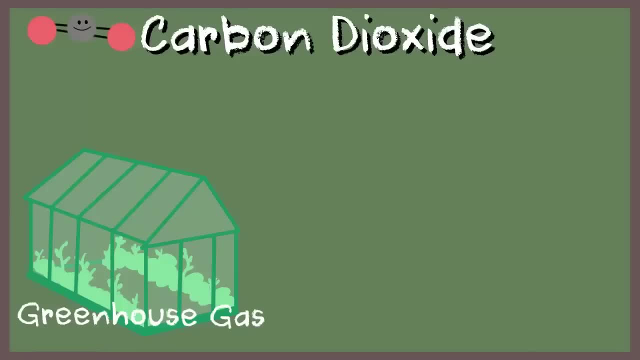 The burning of fossil fuels produces a lot of carbon dioxide, but too much of that leads to the concern of excessive carbon dioxide in the atmosphere. Carbon dioxide is a greenhouse gas, which means that it can trap heat in the atmosphere, So too much carbon dioxide is not a good thing. 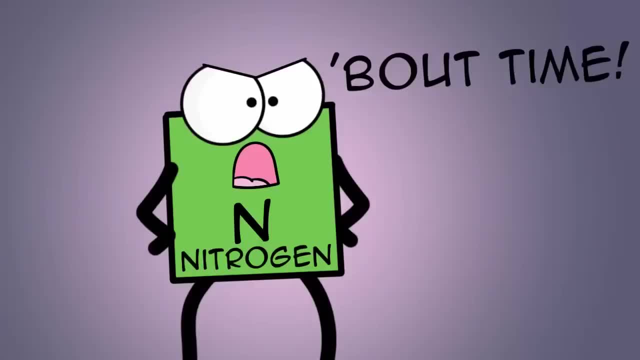 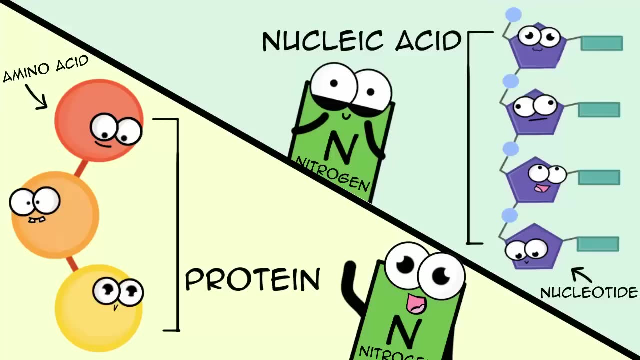 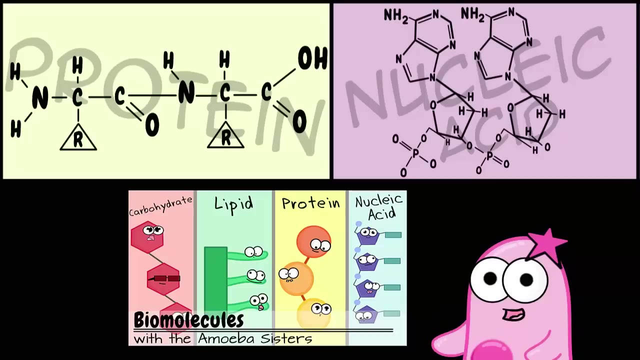 Now, what about nitrogen? Well, nitrogen is a critical element in amino acids- Remember, that's the monomer of proteins- And it's also an element in nucleotides, which are the monomers of nucleic acids. And, if you remember from our biomolecule video, proteins and nucleic acids are two very important. 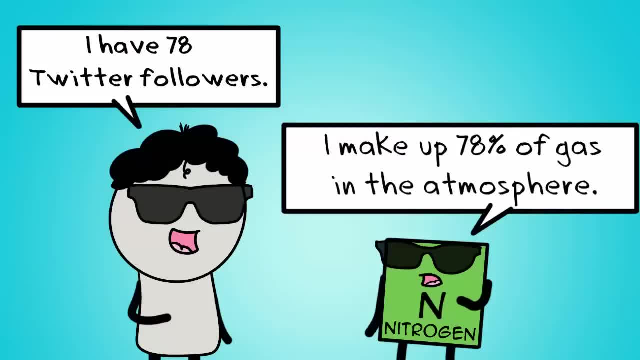 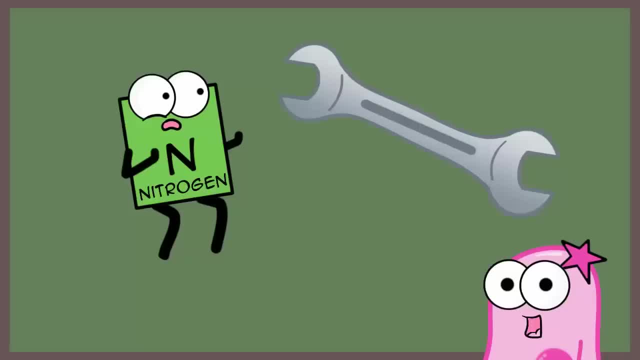 biomolecules for life. Nitrogen is kind of a big deal in the atmosphere, considering it's the primary gas in the atmosphere. The thing about nitrogen is that it's much more useful to organisms when it's fixed and to other, more usable forms. 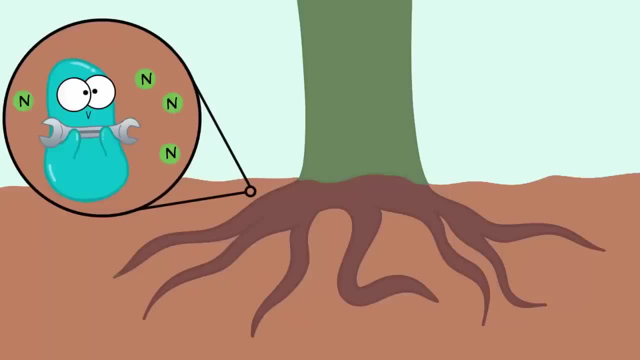 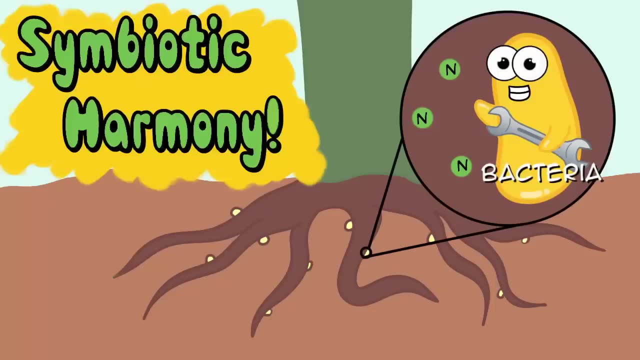 Nitrogen can be fixed by bacteria which could be living in the soil or even in the roots of some types of plants, where the bacteria live in symbiotic harmony inside the roots, Meaning the bacteria get a home in the plant root and the plant gets the benefit of this. 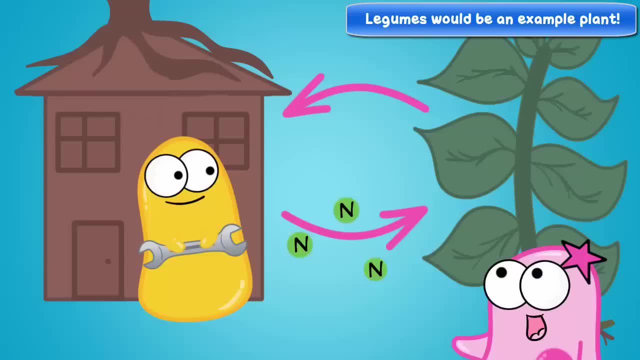 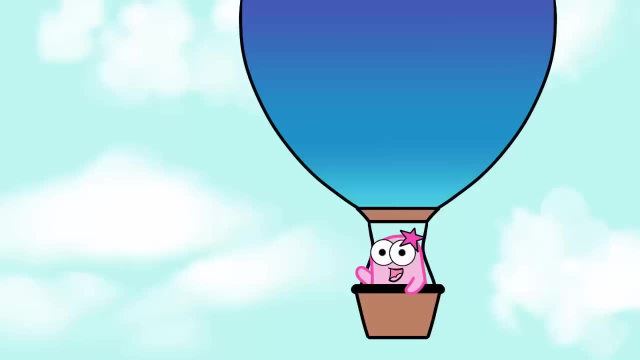 fixed nitrogen. Now, once again, we're just looking at one pathway Here in the nitrogen cycle, So keep that in mind. This is just one way for nitrogen to cycle. OK, so let's take a look at this. nitrogen in the atmosphere. 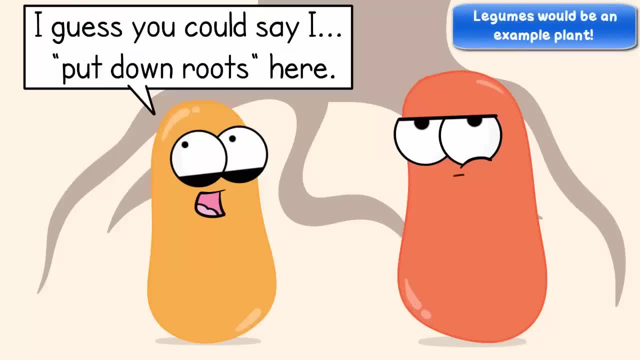 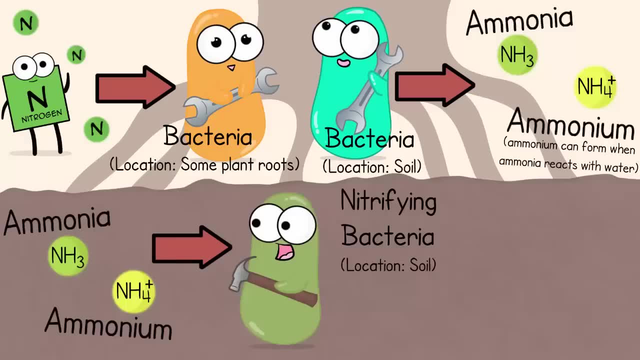 Consider the type of plants that have nitrogen-fixing bacteria living in their roots. The nitrogen is fixed by those bacteria in a form of nitrogen known as ammonia and ammonium Nitrifying bacteria in the soil can convert the ammonium to nitrates and nitrites forms. 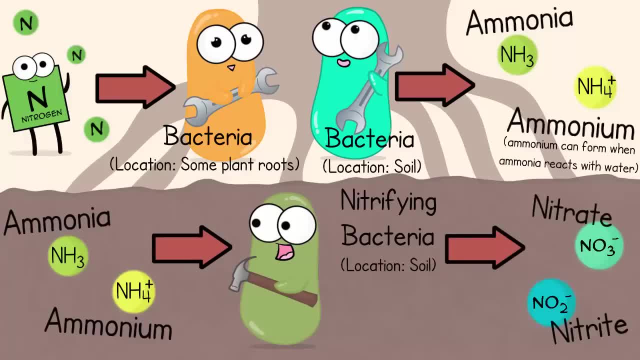 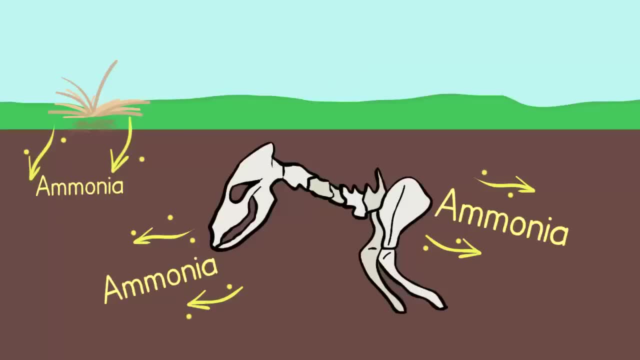 of nitrogen that plants can also easily use and assimilate. Now Animals can eat those plants and obtain that nitrogen When both plants and animals decompose. decomposers return ammonia to the soil in a process called ammonification, where it can be used and reused again. 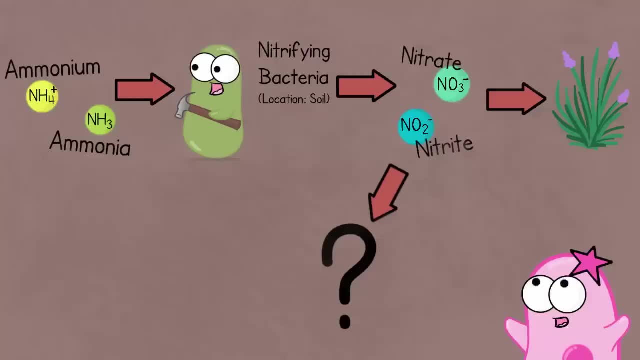 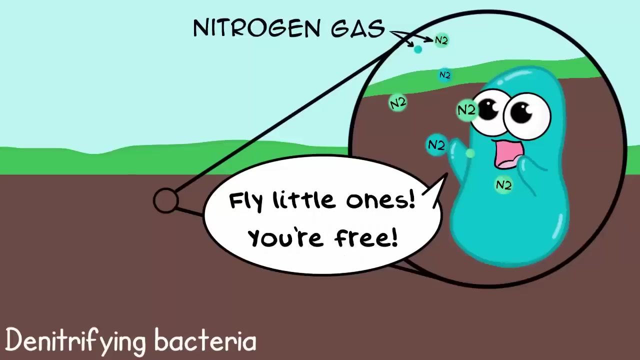 But not all the nitrates and nitrites get assimilated by plants. No, there are other types of bacteria in the soil too. Drum roll, De-nitrifying bacteria And denitrifying bacteria in the soil can convert The nitrates and the nitrites back into atmospheric nitrogen gas. 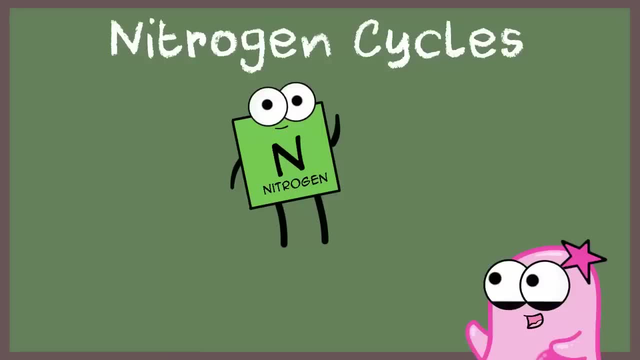 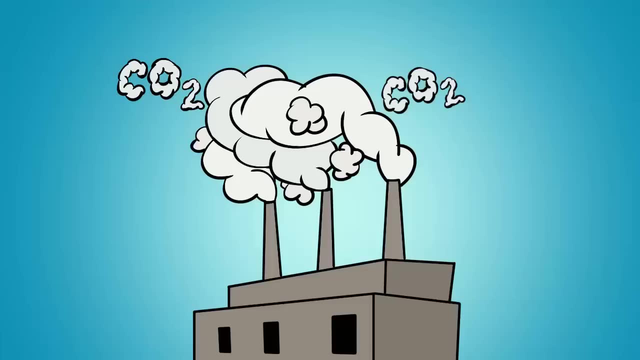 Again, this is one example of nitrogen cycling through. Keep in mind this happens in both aquatic and terrestrial environments, and there are other ways for nitrogen to be fixed and to cycle. You know how we mentioned that too much carbon dioxide can be problematic. You want a balance in these cycles. 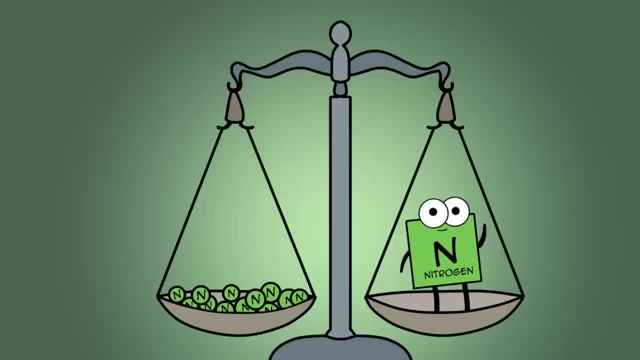 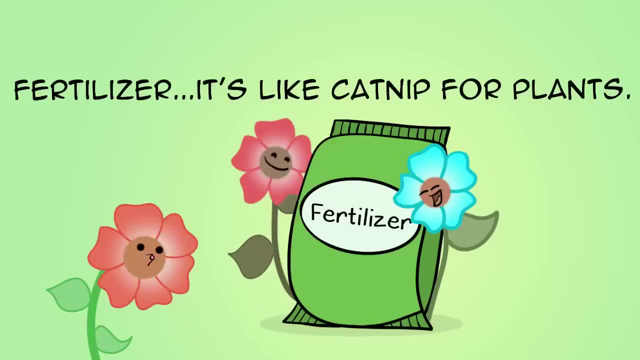 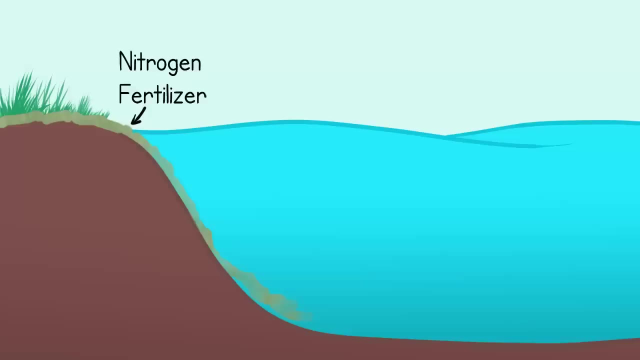 Well, there's a balance for the nitrogen cycle too, and nitrogen pollution can be problematic. Here's one example. Consider plant fertilizer. Plants love it. It contains a form of nitrogen. Well, if it's not used responsibly, the excess nitrogen in fertilizing crops can drain into. 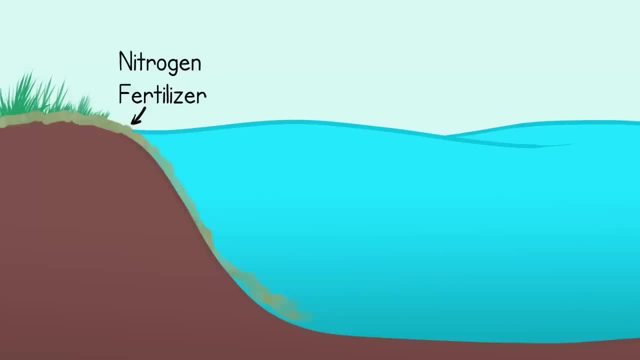 bodies of water, And one reason this could be harmful is that it will basically cause an aquatic producer. heyday, All of the algae and water plants. they now have this crazy load of nitrogen for growth, And that might sound like a good thing. 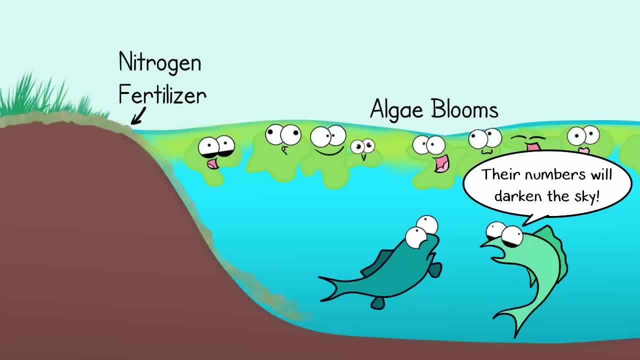 But It can produce excessive growth, It's messy, It can block light to the water And then, when they die and decompose, all that decomposing uses up a lot of dissolved oxygen in the water Which can be harmful to aquatic life. who needs the oxygen? 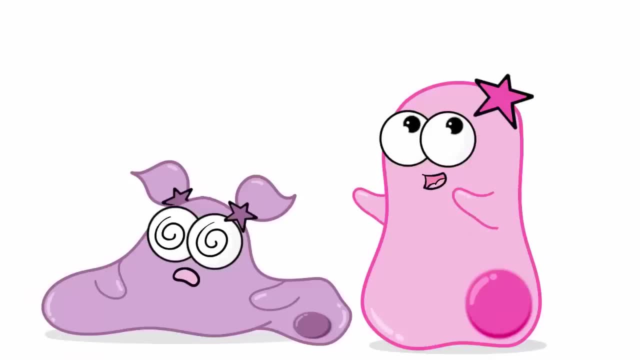 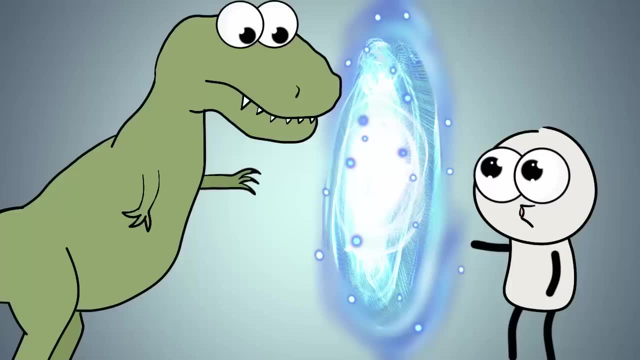 Phew, Now you know this recycling of carbon and nitrogen is pretty remarkable. Just think You could contain a carbon atom that was once part of a dinosaur. Because of all this recycling And the carbon and nitrogen cycle, It's just another beautiful thing connecting all of us.